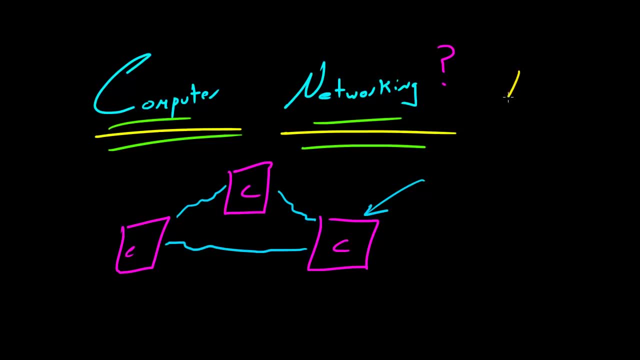 I don't just mean personal computers, I'm talking about cell phones. You know, this is obviously a cell phone, kind of looks like a gun. You can also have a printer. So whenever I say computer, I mean a bunch of different things and, Aside from, you know, just these computers being part of a computer network. 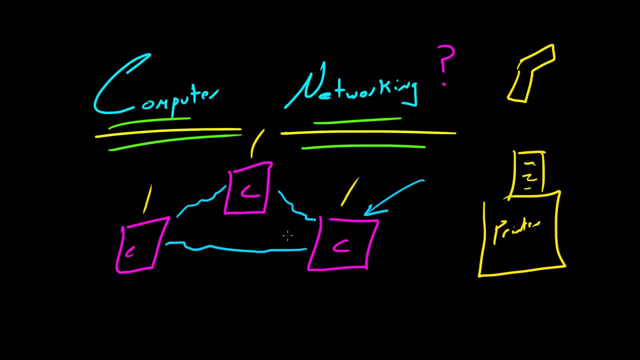 You also have other parts as well, as you guys are going to find out. These computers need a way to communicate with each other and in this little diagram I use, I'll say: this is copper cable, but, as you know, there's also Wi-Fi and, you know, satellites. 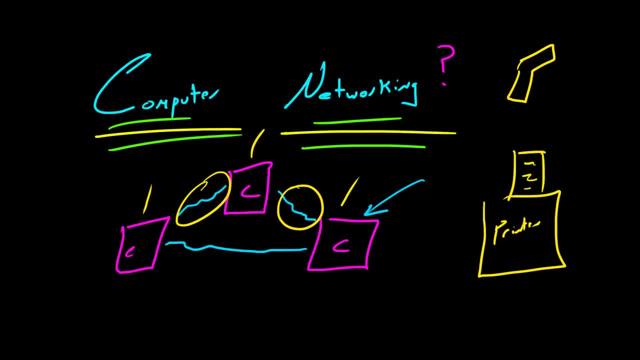 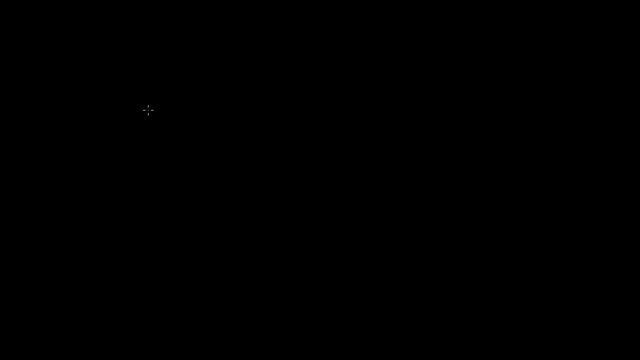 And there are a bunch of different parts that make up an entire computer network, So it isn't just the computers themselves and we're gonna be going over everything. So basically, Let's go ahead and talk a little bit about the copper wire or the Wi-Fi waves. 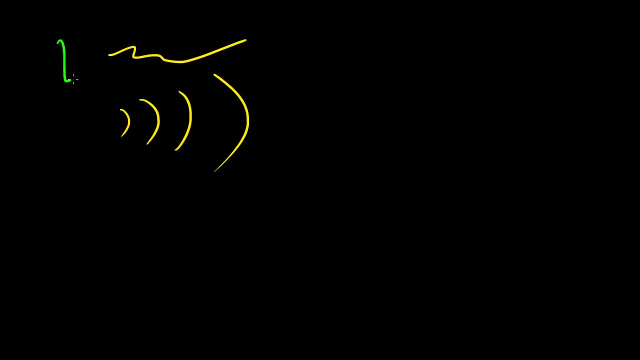 You need this part of a computer network because whenever you connect two computers to each other, They need a way to pretty much transmit data or share data. Just go ahead and write that. so that's basically the purpose of a computer network, because if you just go ahead and connect it a 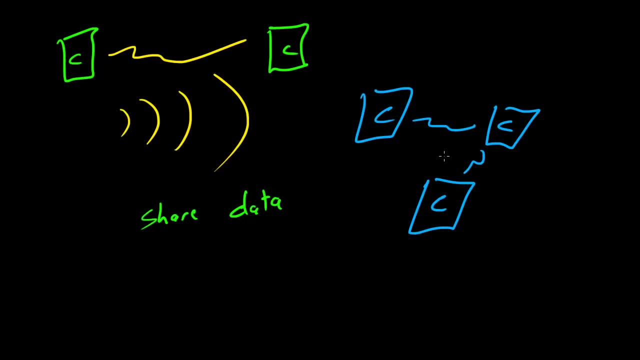 bunch of computers. Okay, this is pretty cool, But why on earth Would you ever want to connect a bunch of computers? Well, the answer is right here to share information, and you do that, Like I said, through copper wire, fiber optics, radio waves- even infrared- and microwaves are used nowadays. 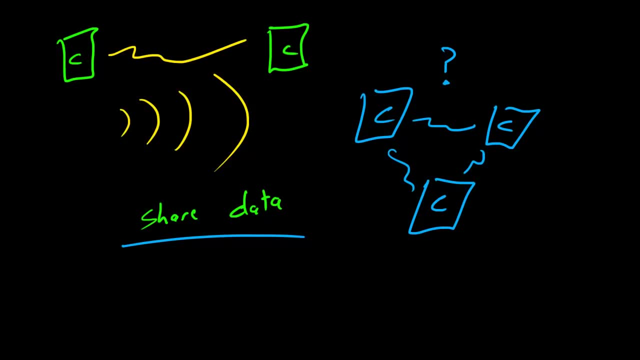 Whenever we're sharing data between computers. so, with that being said, What do I mean by share data? Well, that kind of sounds like you're in a school and you want to, you know, send documents from professor to professor. professor like share and pour in, you know? 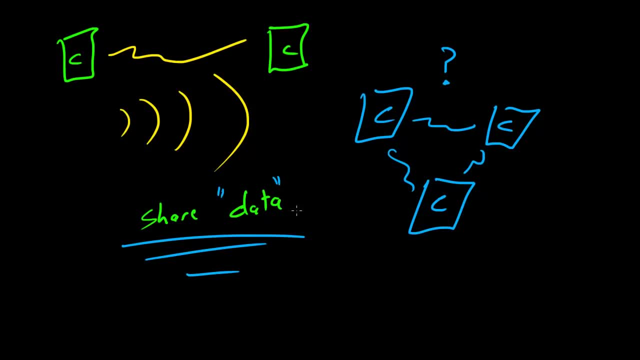 scholarly data. well, data doesn't only mean you know, boring data that you learn in school. it can mean a bunch of different things. the first thing is, of course, like we said, documents. maybe you have, you know, a paper you wrote and you want to send it to another college. you can go ahead and share documents, but 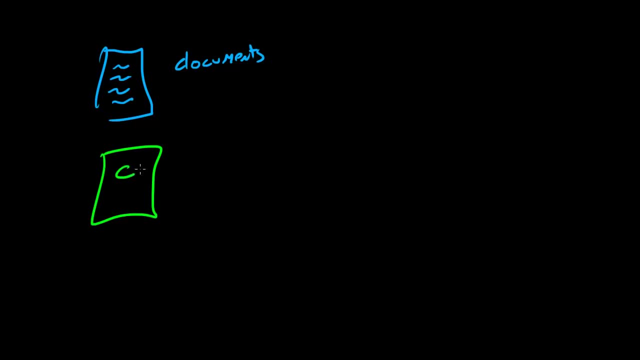 data can also mean stuff like pictures, so let me go ahead and draw a little picture right here. so basically, you can remember, whenever I talk about data, a lot of people just think of. you know documents and boring text, but you can remember. you know pictures and video because if you sign up for a data plan, 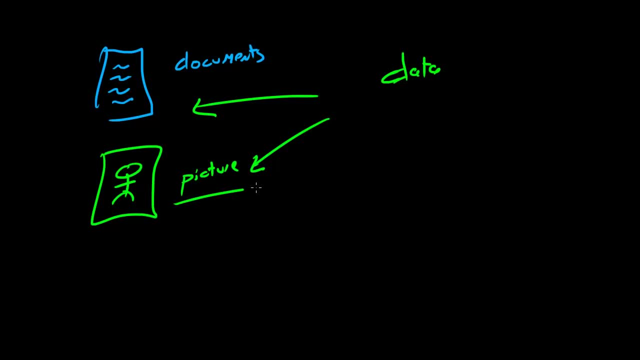 then, of course, what's eating up all your, you know, usage? it's the video, it's the pictures. that's what really gets you and that's why, you know, Verizon is raking in the big bucks right now. so, basically, by data, this is what's transferred in the 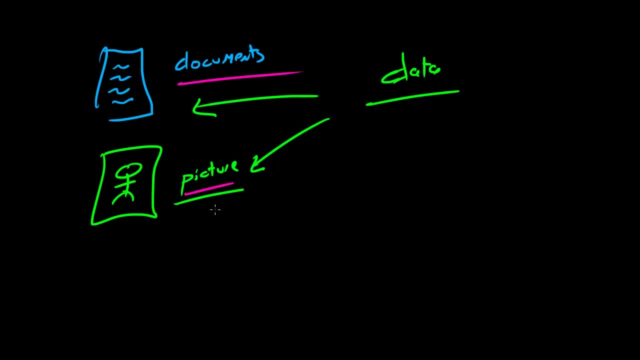 computer network. we have documents, we have pictures. well it's do we have videos? so we'll put a little YouTube player right here, and then we're going to go ahead, and go ahead, and go ahead, and right here. and what kind of videos? well, they're on YouTube or Netflix, by the way. 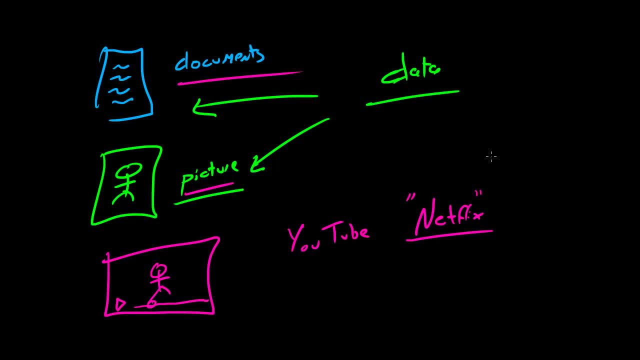 I'm gonna throw a bunch of fun facts that you guys in these tutorials. did you know that Netflix uses or is responsible for almost 32- actually more than 32 percent of the entire bandwidth in the United States? isn't that freaking amazing? and we'll talk about why videos use so. 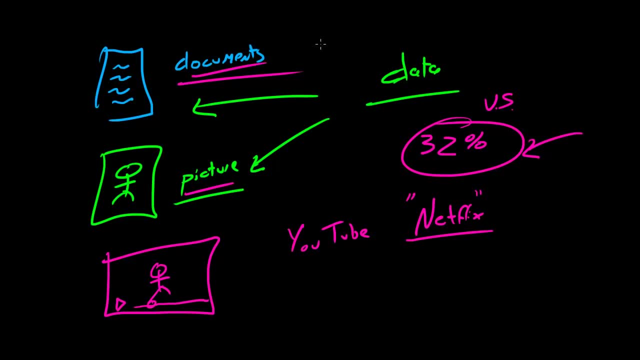 much data, but, anyways, these are the different types of data that we can, you know, transfer computer to computer in a computer network: Netflix videos, YouTube videos, which are basically millions and millions of videos of cats or girls putting on makeup- by the way, girls, why do you need so many tutorials on how to? 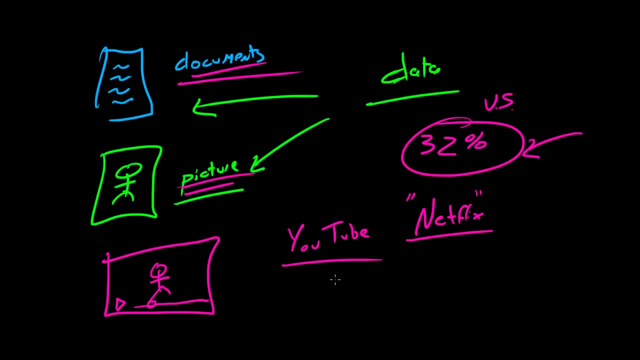 put on makeup. you think if you put it on one way then you know it's the same way forever. but if anyone has an answer to that, then just go ahead and let me know. know. why do girls put on makeup? I don't know, it's a mystery. and of course the biggest computer network it of 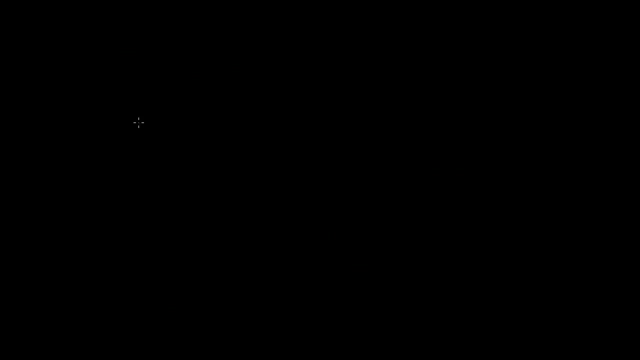 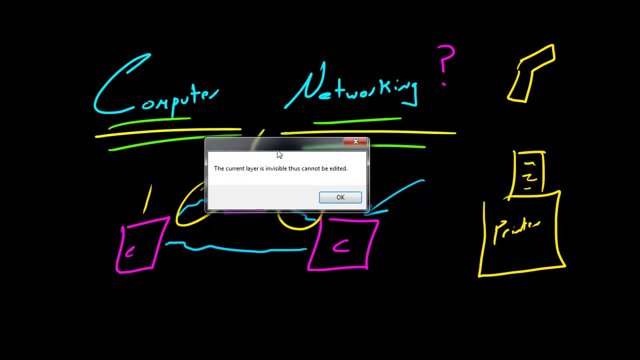 all is the Internet. so that is basically your very first introductory video. let's see what we covered. first of all, what is a computer network? it's based basically a bunch of that's embarrassing- a bunch of computers connected to each other. why would we want to connect a bunch of computers together? yeah, I'm sorry, guys.